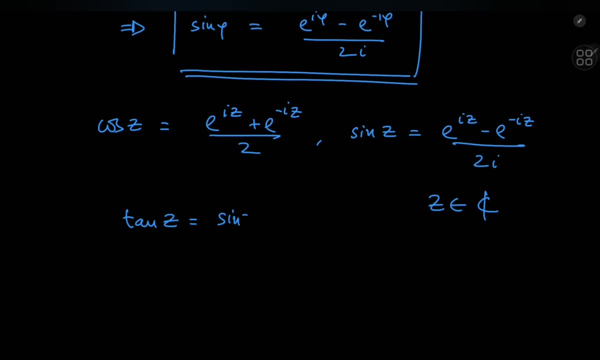 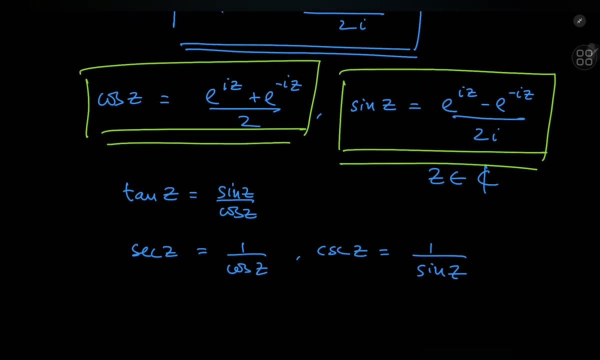 For example, the tangent of z being sine z by cosine z, and the same old definitions for the secant and cosecant functions. Another nice thing here is that you can easily verify, using these definitions, that the trigonometric identities we know all hold in the complex realm too. For example, you can verify that. 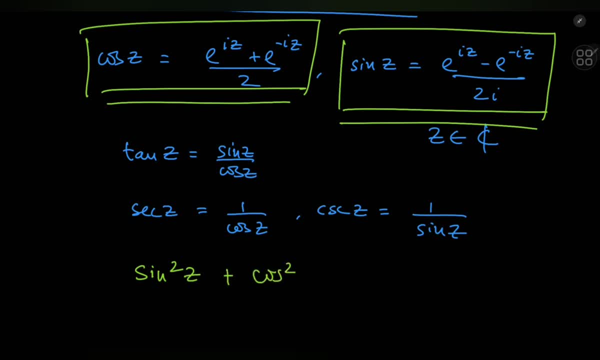 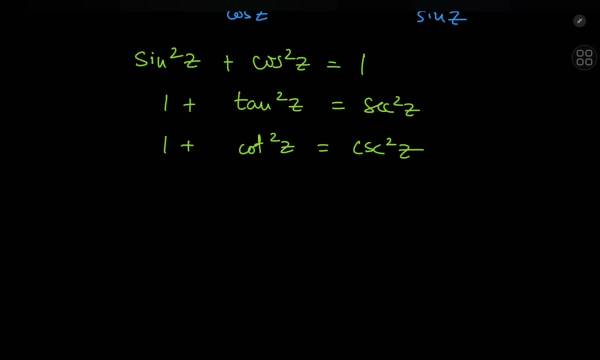 the squared sine of z plus the squared cosine of z equals 1 for all complex numbers, And that, of course, is left as a little exercise to you, the viewer. Now, the complex trigonometric functions are very closely related to the complex hyperbolic trig functions. And how exactly are 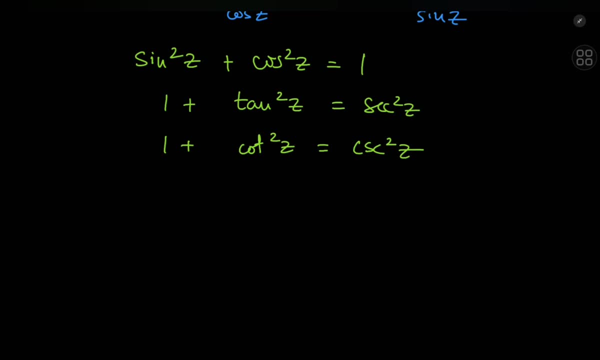 they related. Well, let me show you in a very cool way. So let me take the cosine of z, that is e to the i z plus e to the negative i z divided by 2, and perform a trigonometric analysis So we can. 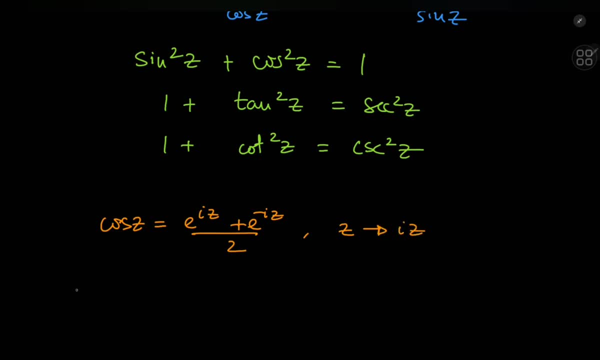 see that the trigonometric functions are very closely related to the complex hyperbolic trigons. So in that case i get cosine i z equal to e to the i times i z, which of course is e to the i squared z, and i squared is just negative 1. so we have e to the negative z plus e to the z. 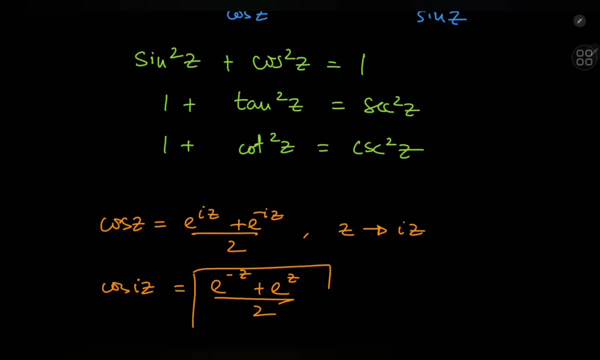 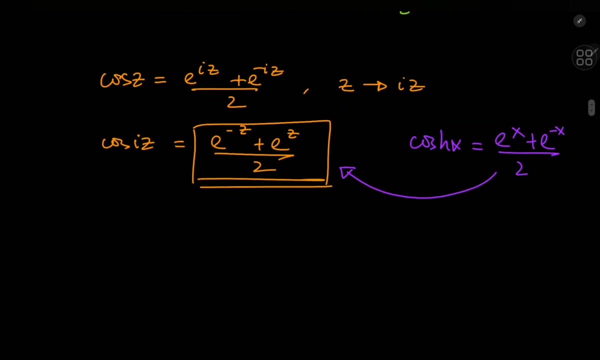 divided by 2.. Now pause at this structure and take a moment to recall exactly how we defined the hyperbolic cosine. So cos x is defined as e to the x plus e to the negative x by 2.. So, keeping with the structure for our complex valued hyperbolic function, we see that the cosine of i times z 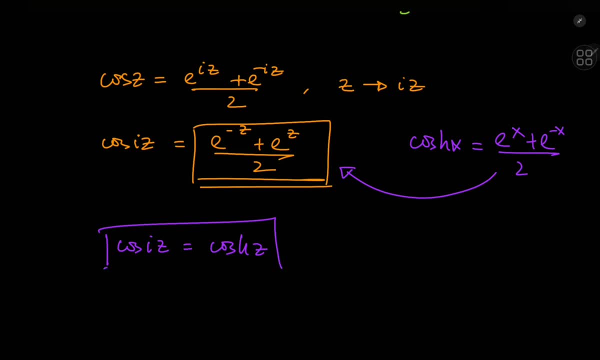 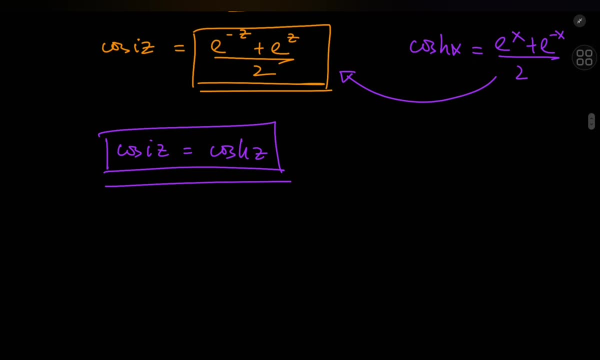 equals the cos of z, which is a pretty cool relation. Similarly, we can figure out the relation between the sine and the hyperbolic sine, or the sin of z. So sine z equals e to the i z minus e to the i z divided by 2i. Again the same transformation from. 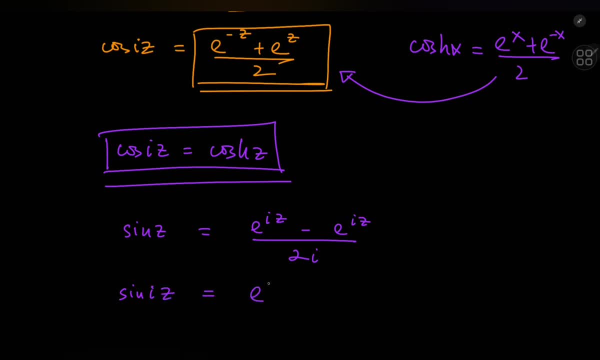 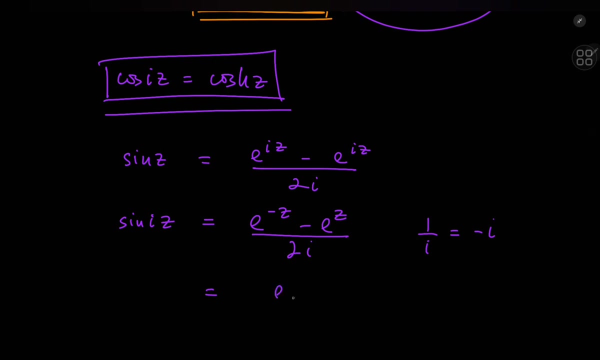 the z realm to the i z realm gives us e to the negative z minus e to the z divided by 2 times i. Now division by i is the same as multiplication by negative i, so that means i can write this as e to the z minus e to the negative i. So that means i can write this as e to the z minus e to the i z divided by 2i. 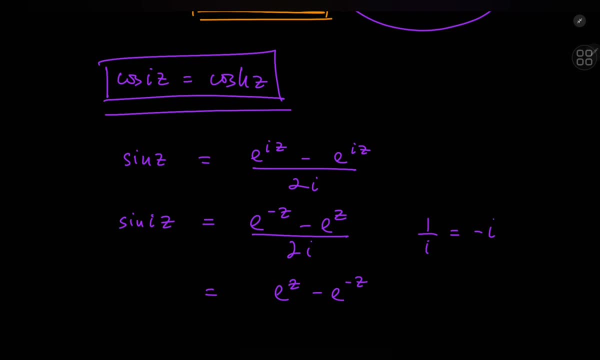 a negative z, where I switched up the order in the numerator to get rid of this extra negative sign that I would have introduced, And we have to divide this by 2 and multiply by i. Now this looks exactly how the sinch function should be defined, recalling its definition from the real 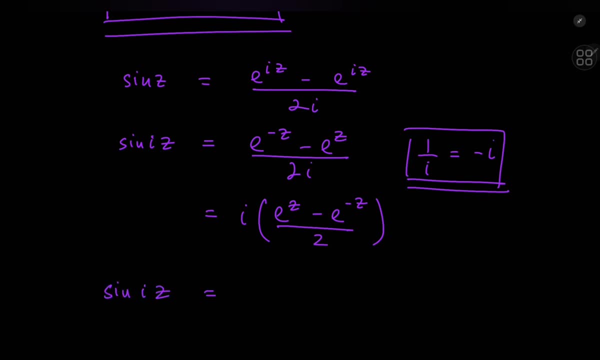 realm. So we have the sine of i times z being equal to i times the sinch of z, And both of these equations- the ones for the Cauchy and the sinch functions- implies that the hyperbolic tangent, the tangent of i z, equals i times the hyperbolic tangent of z. Now this length of a 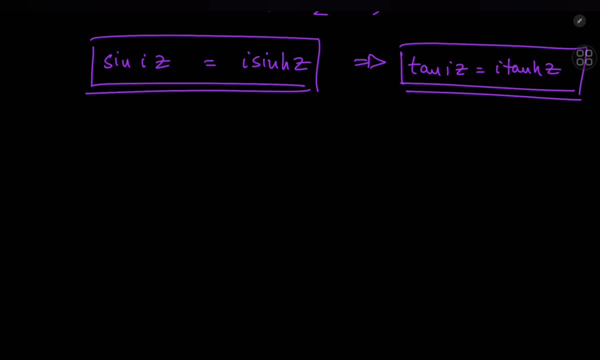 circular and hyperbolic trigonometric functions is pretty cool, but it's not the only way in which the complex trigonometric functions set themselves apart from their real valued counterparts. Another marked distinction is the fact that the complex trig functions are not bounded Now bear. 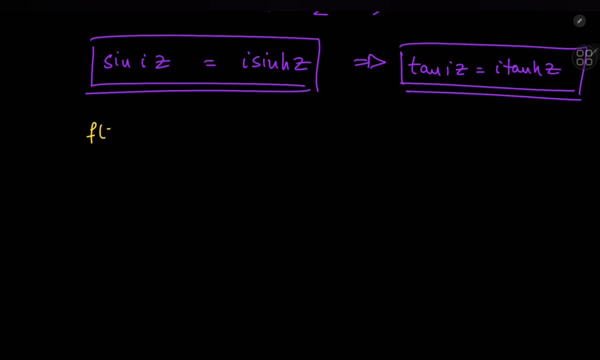 in mind. we're talking about complex valued functions here. So if I say that f of z is bounded, I mean its absolute value is bounded, So the complex trig functions are not bounded as in. if I were to write an equation like sine x equal to 2 and I were to task everyone with 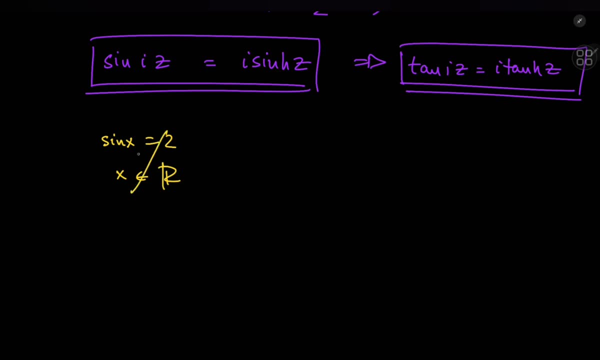 finding a real number that satisfies this equation. that's not going to happen. It's invalid in the real realm that is. However, in the complex realm, it's quite easy to find a complex number, z, satisfying this equation. And how are we going to do that? Let me give you a nice demonstration. 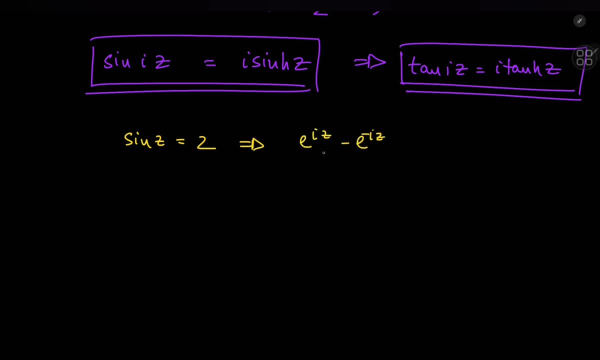 We have e to the i z minus e to the negative i z. divided by 2, i equal to 2.. So this implies that we have e to the i z minus e to the negative i z equal to 2 i i Now. this equation is: 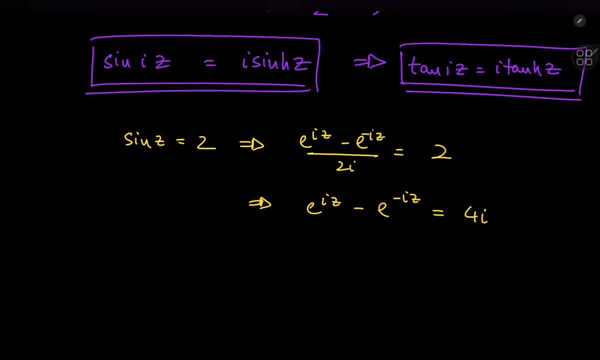 satisfied. So we have e to the i z minus e to the negative i z equal to 2, i i Now, if we're able to, to 4 times i. so expanding using e to the i z would give us a very nice structure. it would give us e to: 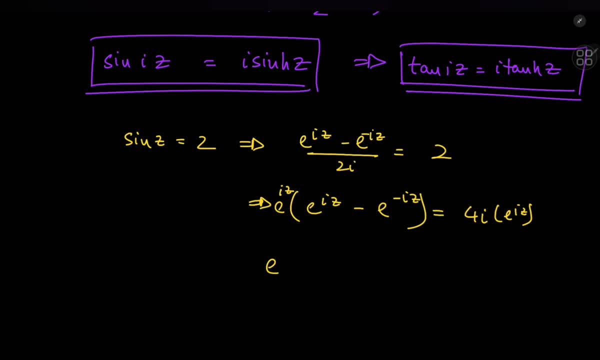 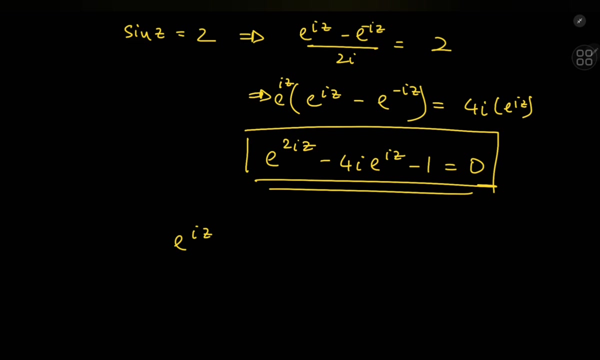 the 2 i z. wait, let me just fix that. yeah, much better. minus 4 i times e to the i z. minus 1 equal to 0, which is a quadratic equation in e to the i z, and we can solve this using the quadratic formula: as e to the i z being equal to 4 i plus or minus square root, the square of 4 i is negative. 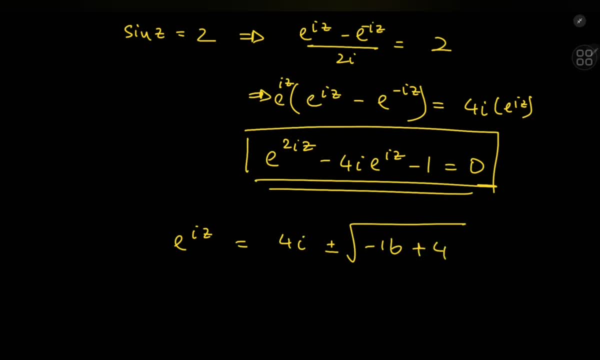 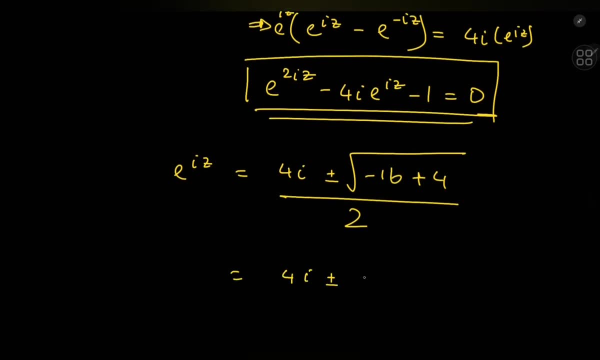 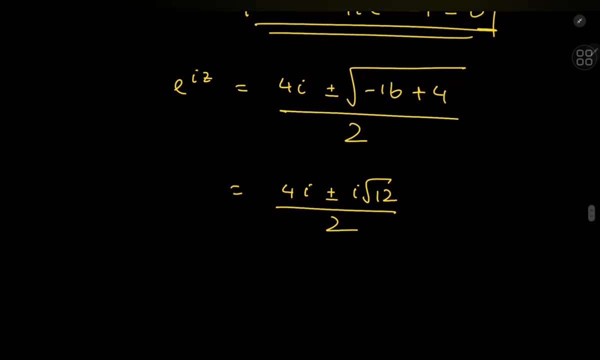 16 minus, but we got a plus sign now- and 4- yeah, that's right- divided by 2. so what we get is 4 i plus or minus negative. 12 in the square root basically means i times 12 divided by 2, so we have. 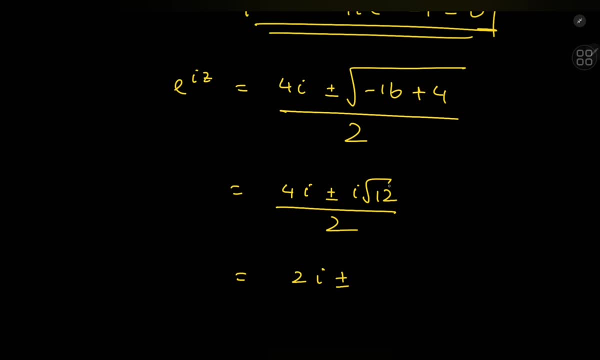 2 i, so we have 2 i, so we have 2 i plus or minus. this. 12 can be the square root. 12 can be written as 2 times root 3, right, so we have i times root 3 as well, and this equals e to the i z. 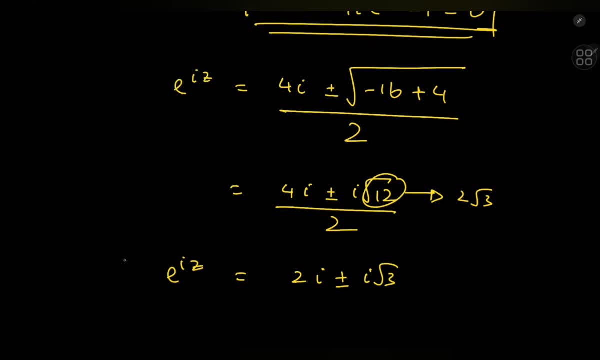 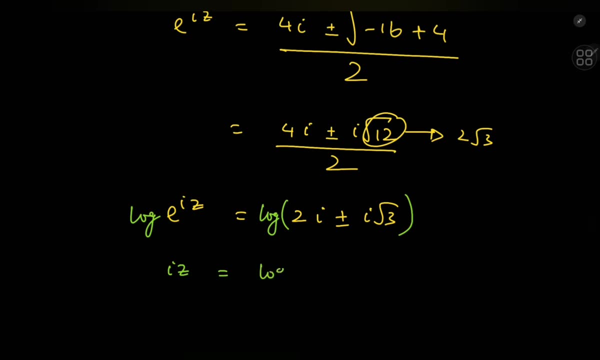 now, to get z, we can use logarithms. so using the complex logarithm we have i z equal to the logarithm of i times 2 plus or minus root 3, and of course we can expand. now to get z, we can use the Incorporated Error. 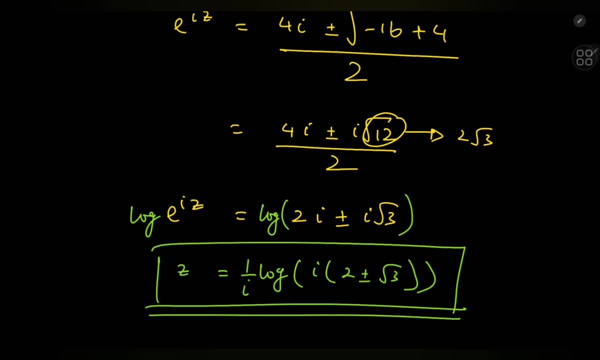 remember we have a problem. if i times z is equal to i z. i looks like that. so we need a double family. so ever since we рассted all numbers on Z, we only get z less than or equal to. let's say, z minus 8a is equal to 3a plus i minus 1. so even though we did not use larger 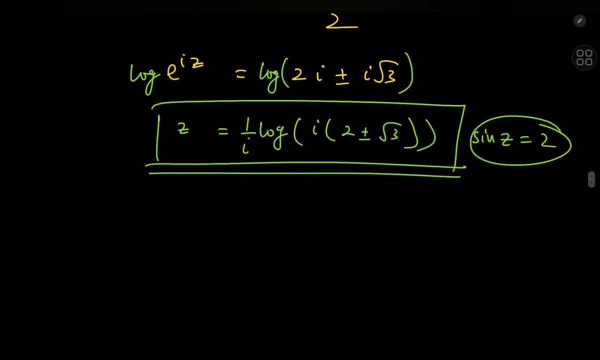 values. we only do it into smaller Working Skills. so we know that i minus 2 equal to z, is equal to i 2 minus some two. we must do: if i feels greater than or equal to the n, we just do it f one over 2 by e to the i, and now we can bring this to the assembly. 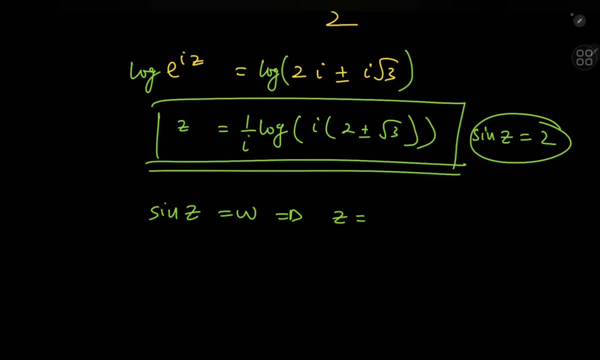 the cama, I would get z equal to 1 by i times the logarithm of i w plus or minus square root, 1 minus z squared. So we see a problem here with the logarithm function. This is a multi-valued function, so that means z which, according to this equation, should be defined as the inverse. 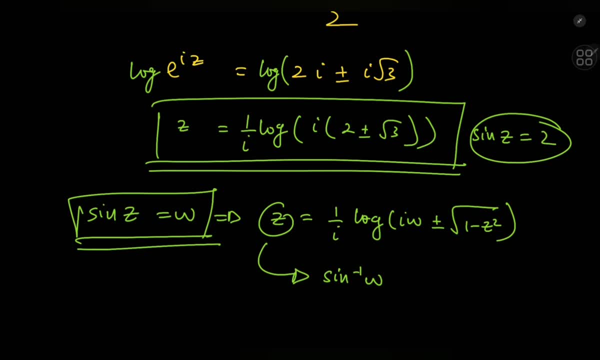 sine of w is not a continuous function. So how do we solve this problem? Well, obviously, we're going to need to define branch cuts, Branch cuts to take care of the logarithm and, of course, specify which branch of the square root function we're using. 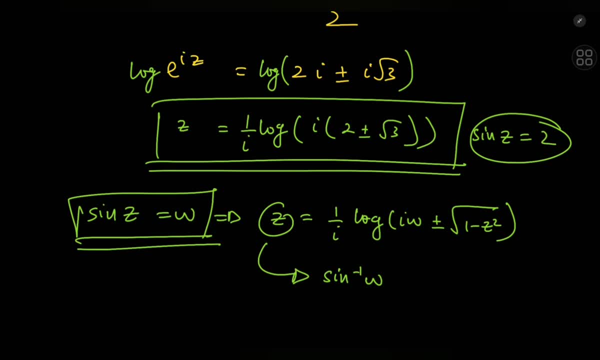 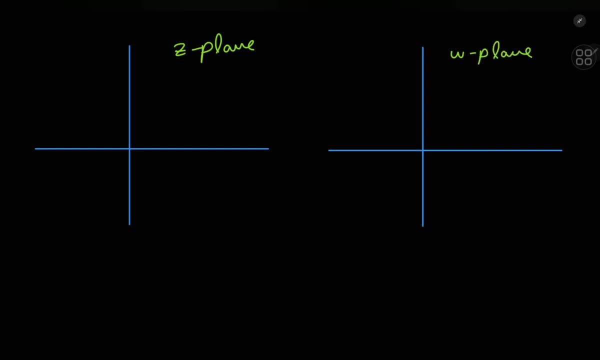 And to achieve all of that we're going to need a couple of complex planes. So here's my z plane and w plane, And we translate from z plane to w plane using sine z equals w. Now let's analyze what happens to the complex. 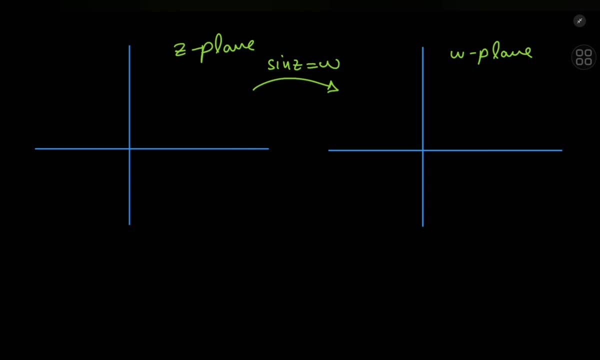 numbers in the z plane. under the transformation, sine z equal to w when I let the imaginary part of z be 0.. And why is this so important? Why is this case so important? Well, if the imaginary part is 0, it implies that sine z is 0.. And if the imaginary part is 0, it implies that sine z is 0. 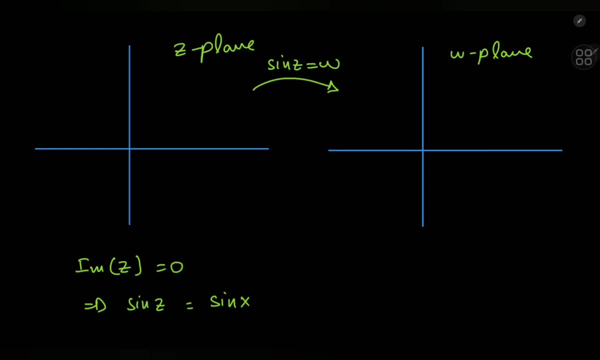 So the value of the real number is just the real value of the sine function, which we know is bound between positive and negative 1.. So what this means is that the entire real axis in the z plane is mapped onto the segment of the real axis in the w plane between negative and positive 1,. 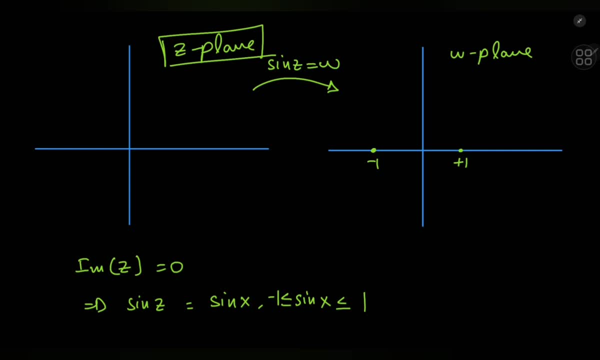 which is the real value of the sine function. So the real value of the sine function is just the real value of the sine function And the FAR is pretty cool. but besides being cool, it gives us some intuitive reasoning as to how our branch cuts should be defined. 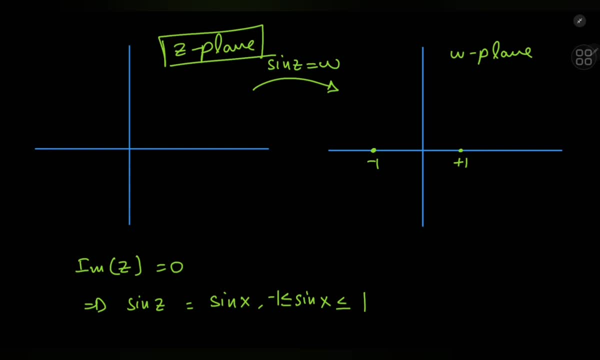 So a nice way to define them here would be to exclude all those real numbers less than negative 1 and even equal to negative 1, because this is a branch point, so let's just exclude it. And we're also excluding all those real numbers greater than or equal to positive 1.. 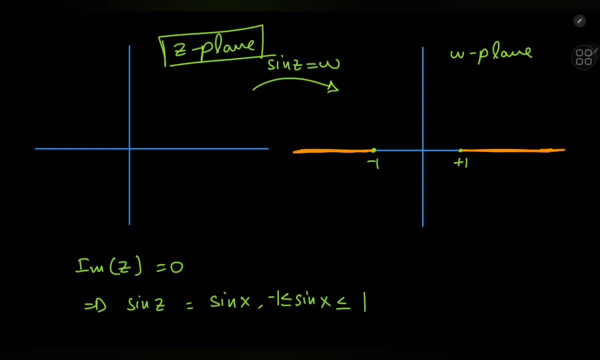 Okay, so those are the branch cuts we needed, and now let's analyze what happens to the strip. bound by x equals negative pi by 2, and x equals positive pi by 2.. Okay, so we see that the real parts of all complex numbers in here are bound between: 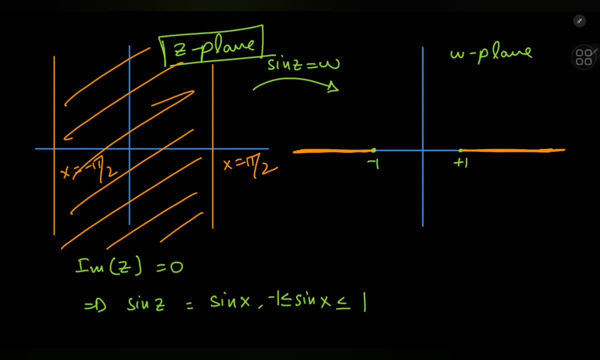 positive and negative pi by 2, whereas the imaginary part is not bounded. So how does the sine function behave under such circumstances? Well, we have sine z equal to sine of x plus i times y, and we can expand this using the classic formula for sine of one number plus another number. 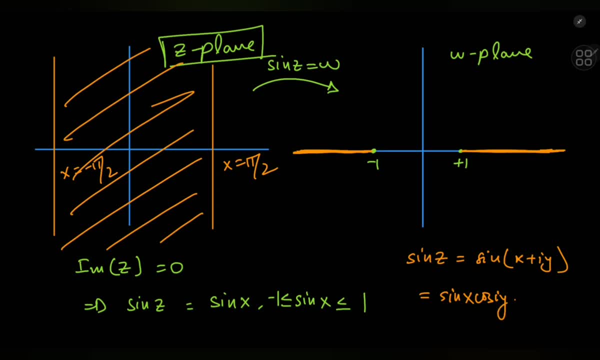 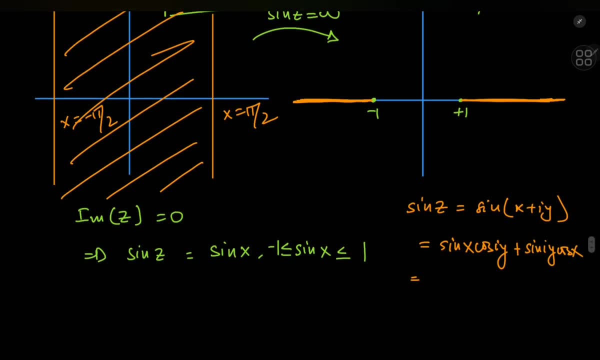 So we're going to have sine x times the cosine of i- y plus the sine of i? y times the cosine of i- y. Okay, so we're going to have sine x times the cosine of i- y plus the sine of i? y times the cosine of x, and cosine i- y is just the cosh of y, so we have sine x times the cosh. 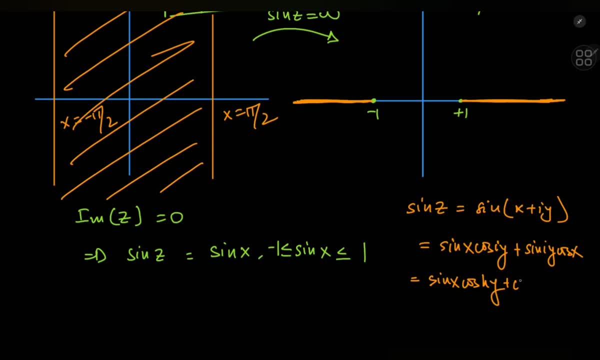 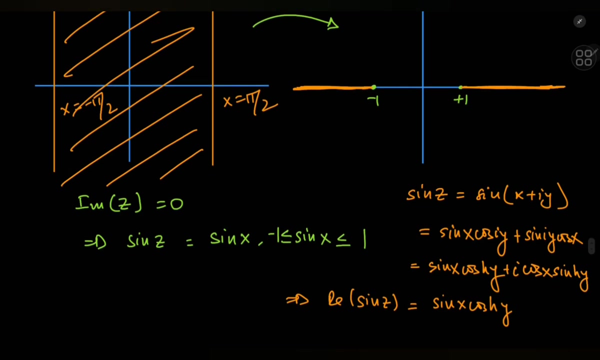 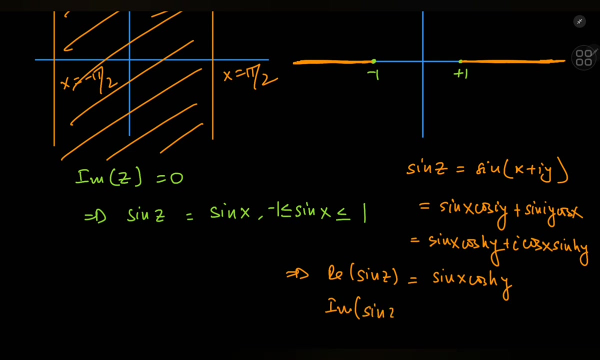 of y plus sine of i. y is i times the sinh of y, so we have i times cosine x times the sinh of y. So this implies that the real part of sine z equals sine x times the cosh of y, whereas the imaginary part of sine z is cosine x times the sinh of y. and while we've bounded x, 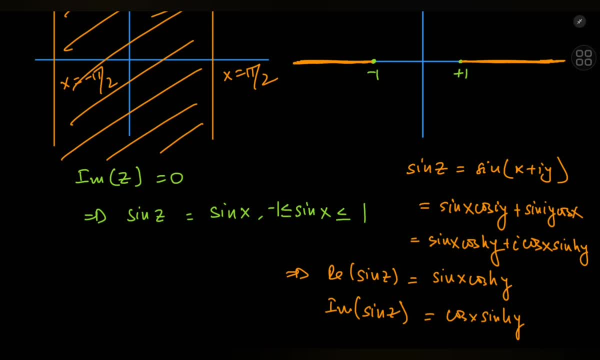 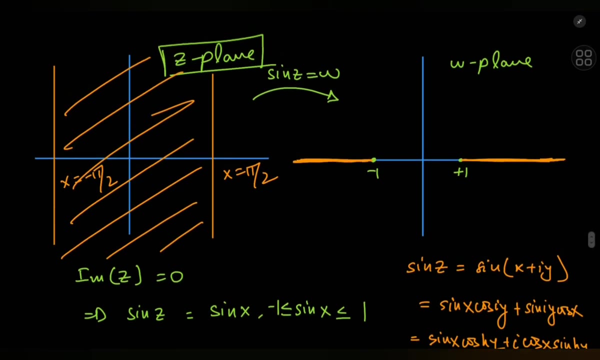 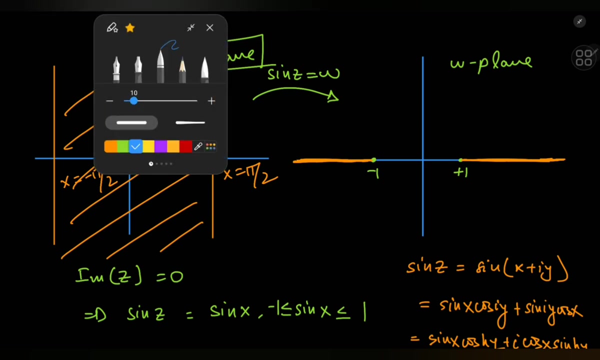 to lie between negative and positive pi by 2, we've left the y variable unhinged. So because we have hyperbolic functions over here, we're going to cover all possible values for the real and imaginary parts in the complex plane. So that means our strip bound between positive and negative pi by 2, this vertical strip. 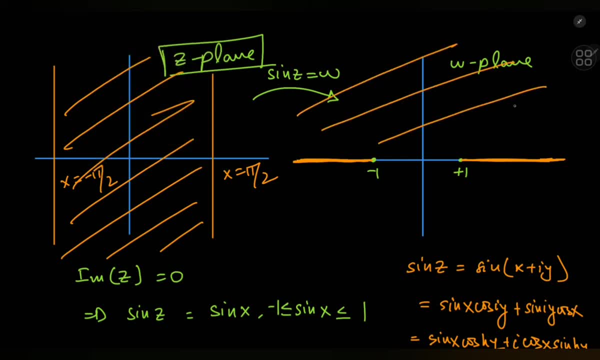 is mapped onto the slit plane, mind the branch cuts. It's mapped onto the slit plane, defined as the complex plane excluding the interval negative infinity to negative 1, as well as the interval plus 1 to wait. this one's included.